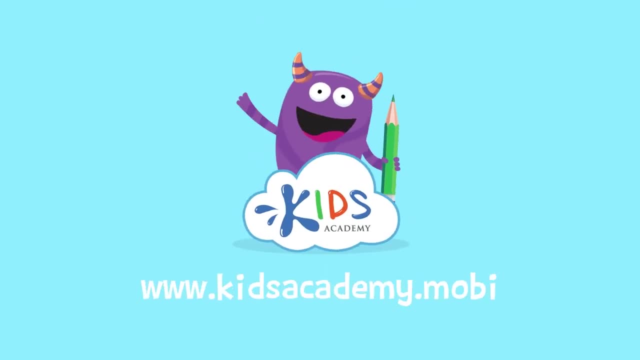 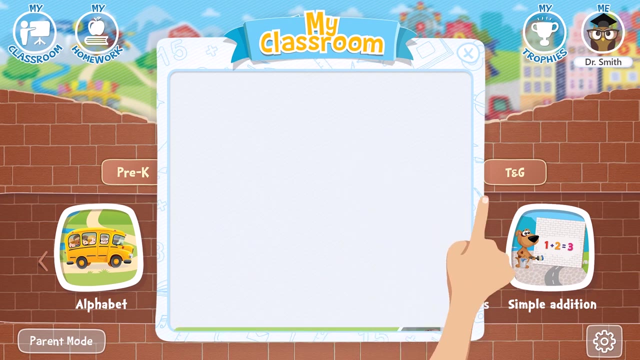 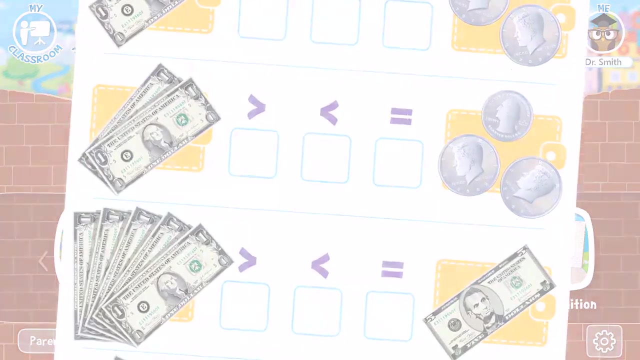 Welcome to kidsacademymobi. Hello everyone, Let's open the worksheet. Don't forget to like this video and subscribe to our channel. You can find the link to this app in comments below. We have a new worksheet today and we're going to be dealing with money. 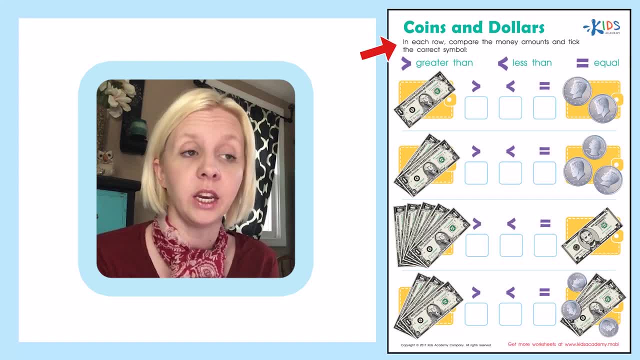 The name of our worksheet is called Coins and Dollars. In each row, compare the money amount and tick the correct symbol. The word tick means just kind of put a check mark there. So what we're going to do is we're going to look at our money on both sides of the worksheet. 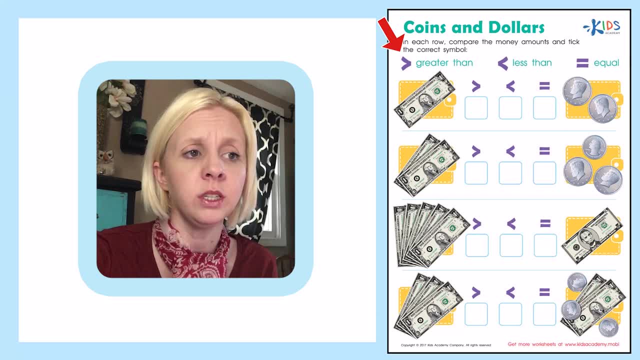 and we're going to decide: is it greater than which is a symbol that looks like this? is it less than a symbol that looks like this? or is it equals to? And you might remember, from a long time ago, we kind of learned that the greater than sign and the less than sign. 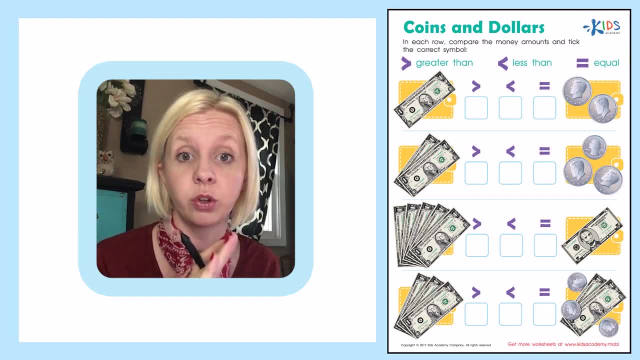 it's kind of like an alligator and it always wants to eat the bigger number, So the less the open part is going to be facing the biggest number out of these here, And then equals means that they're the same amount. So let's go ahead and start on this first one. This: 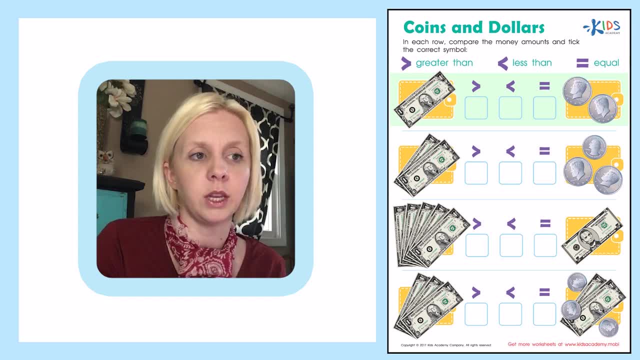 first one is a dollar bill, So we know that the amount for this one is going to be one dollar, and I'm actually going to write this over to the side. I've got one dollar right over here. Then over on this side we have two fifty cent pieces or half dollars. So 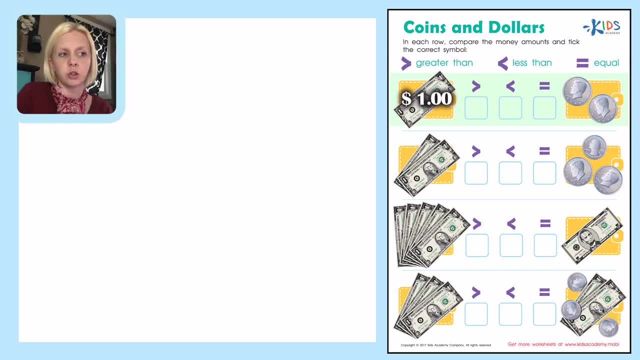 fifty plus a dollar equals one dollar, So we're going to write this over to the side. So this is fifty. We might already know what that is, but let's just write it out to the side. Fifty cents plus fifty cents, Zero plus zero is zero, And then five plus five is ten. 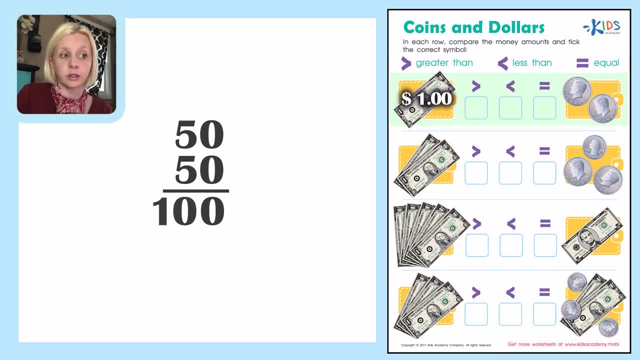 And this actually becomes a hundred cents, which is a dollar. This is like one dollar, So we're going to go ahead and put this over to the side. This is one dollar. So is it? is this number bigger, or is this number bigger, or are they equal to each other? Well, a dollar. 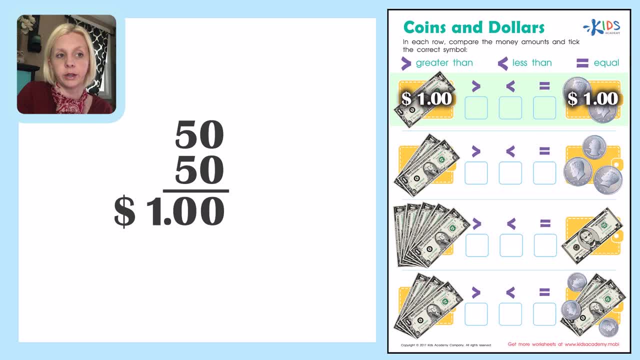 is the same as or equal to a dollar. So I'm going to put a tick mark right here next to the equal sign, because they're both equal. So let's go down to the next one. The next one: here we've got two dollar bills, Okay, So we're just going to write that out: Two. 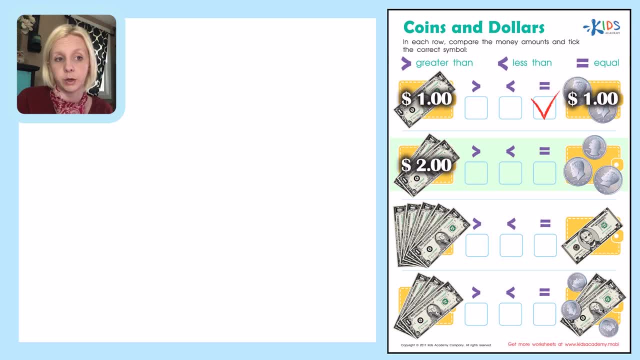 dollars, All right. And then this one over here. we have two fifty cent pieces and a twenty five cent piece. Two fifty cent pieces and add them together. We already actually did this one. So what was the answer to that one? Well, we know that it was a dollar, right? So we have a. 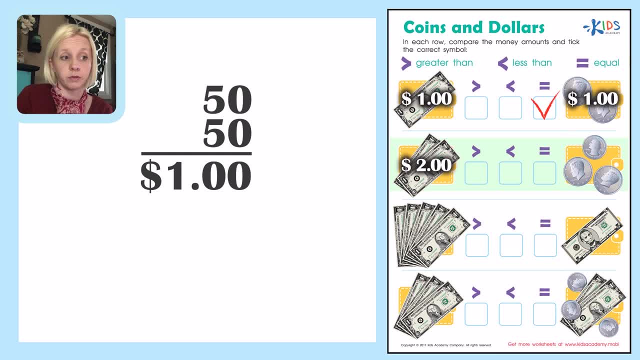 dollar and now we need to add on what? Twenty five cents. So we're going to come over here and add that to the side And remember to line it up, because it's cents, The decimal is actually before it. Okay, So over here we're going to add it up. We've got zero plus. 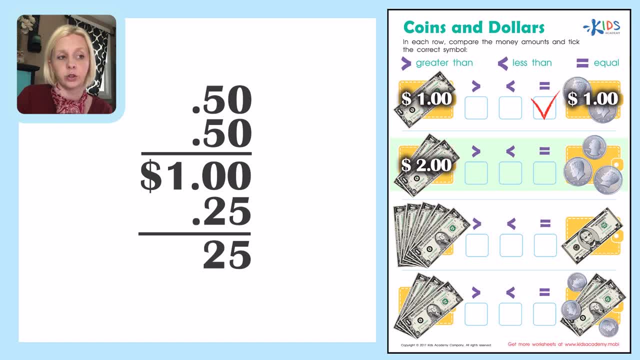 five is five and zero plus two, which is two. And then don't forget to bring down your decimal point. and then a dollar. So this is actually going to be a dollar twenty five. Okay, Which is greater, Two dollars or a dollar twenty? 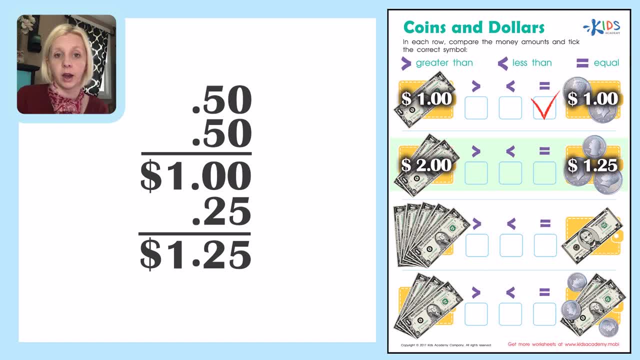 five? The answer is going to be two dollars. So we're going to make that sign face or eat, if you'll call it the bigger number. So it's going to be this one right over here. It's going to eat this and we call that a greater than sign. Okay, All right, Go ahead and write. 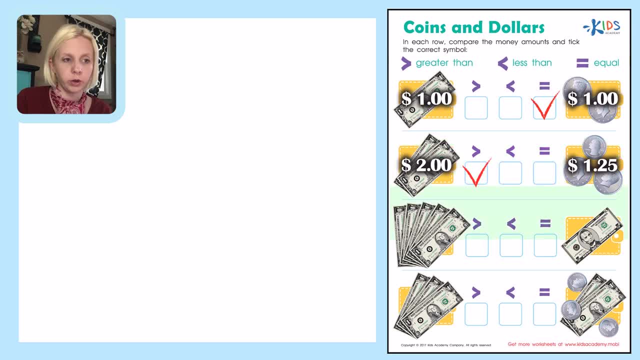 that down, All right, Go down to the next one, The next one. we can count these up. We've got one, two, three, four, five. So over here this equals five dollars, All right. And then over here, if you look up close. 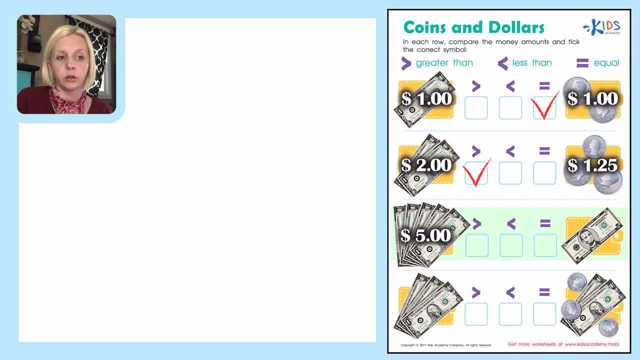 this is a five dollar bill. Okay, So this also equals five dollars. So are is this one bigger or is this one bigger? Are they equal to each other? Well, five is equal or the same as five. So we're going to put our check mark right there. We're almost done. Great job, Let's go down to the last one. 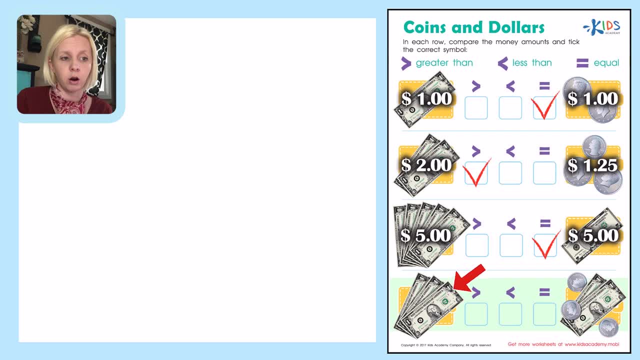 The last one is one, two, three dollars. So we're going to write that out right over here. We've got three dollars, And then over here we can see that there's two dollars, but then there's also some money that we need to add on. So I'm going to write this out to the side. 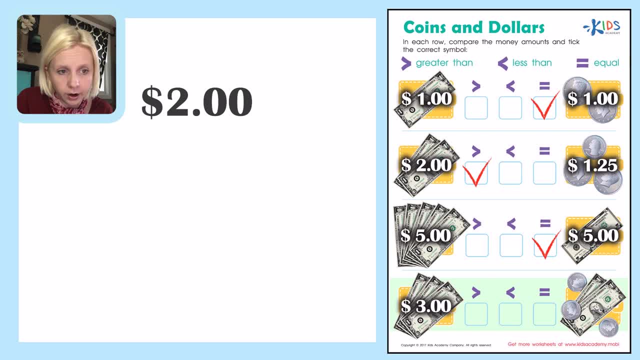 We've got two dollars. Now let's add up our money. What do we have here? It looks like we have one, two, three dimes. Those are all equal to ten cents. So we're going to add ten cents plus ten cents plus ten. 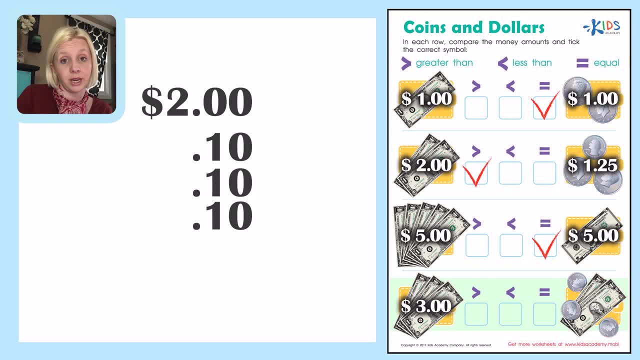 cents And we can add them all up together, or we can actually count by tens. I bet you've done this in the past, So let's go ahead and just count by tens to figure out what just the cents are. So ten, twenty, thirty, So all of this is. 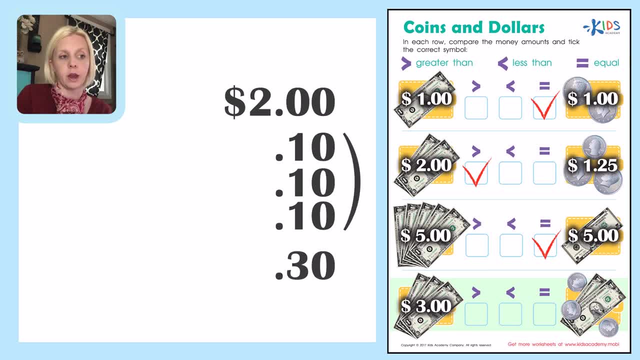 going to be equal to thirty cents, Okay, And I'm going to add that on to my two dollars, And actually this is pretty easy, since it's nothing over here. We're going to take two and we're going to add it to our. 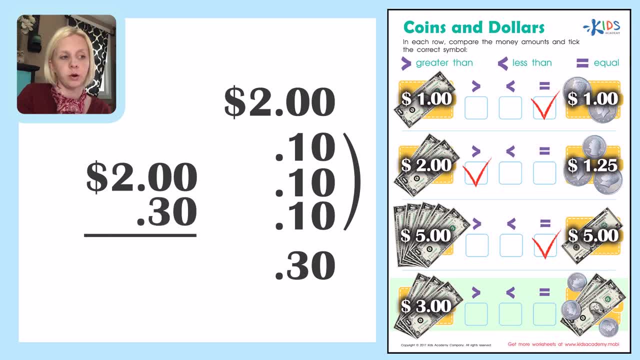 thirty cents. Add them up together. So zero plus zero is zero. Zero plus three is three. Carry your decimal, Bring your two down and we have two dollars and thirty cents. We're going to write that over here: Two dollars and thirty cents. So let's go back. What are we looking for? We're. 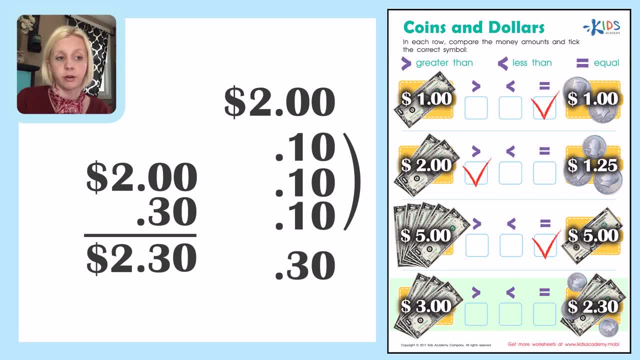 looking for the sign. So which one is greater? Is it three dollars Or two dollars and thirty cents? We know that the three dollars is bigger or greater than two dollars and thirty cents, So we're actually going to put our mark right here. 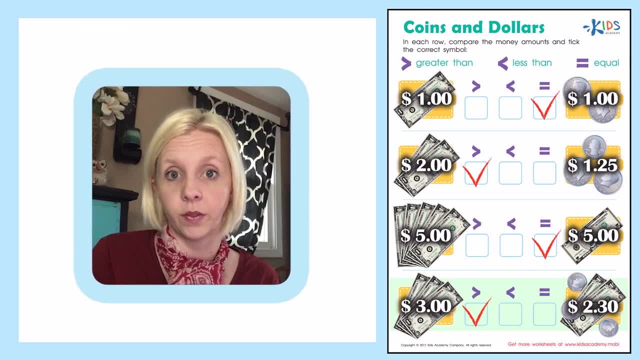 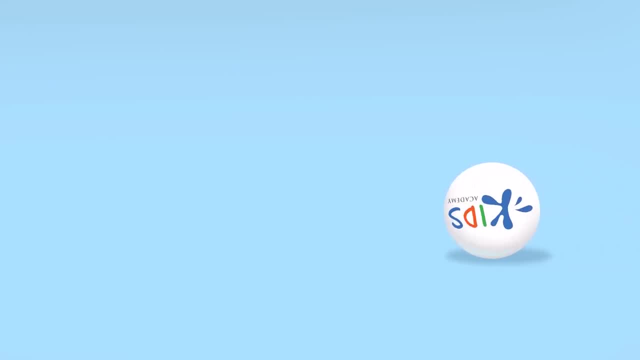 on the greater than sign, since we want it to eat or face the one that's bigger. So nice job. today We are finished. Great work Thanks to our apps and comments below.